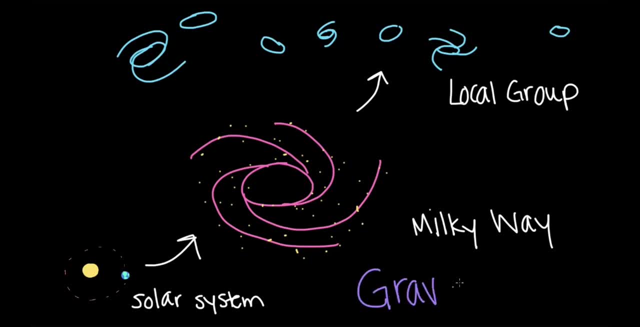 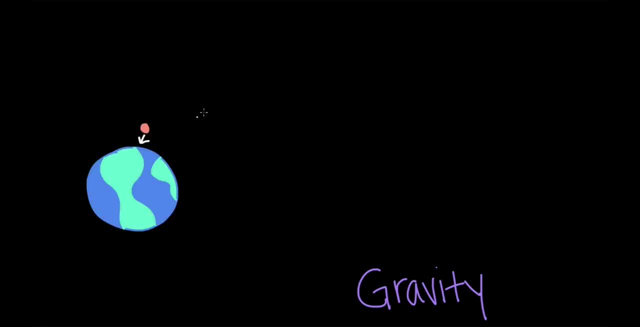 massive groups and clusters of galaxies. Gravity: This is the same as the gravity that makes a ball fall back to the ground when you toss it up into the air. Gravity is a force that operates between two objects that have mass and tries to pull them closer together, whether those objects are a ball. 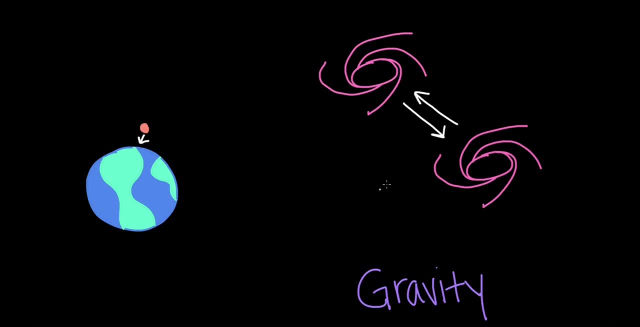 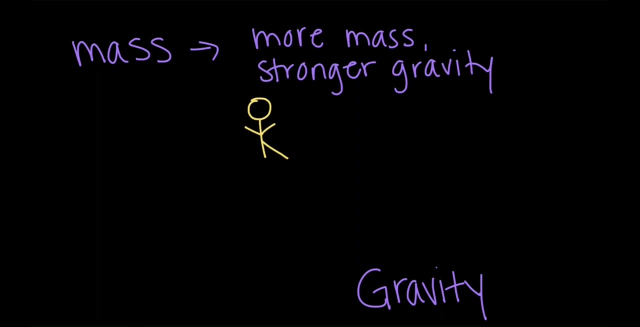 in the Earth or two galaxies. Now the strength of this pull depends on two things. First is the mass of both objects. So as either object gets more massive, the strength of gravity increases. For example, you have a lot more mass than a ball, So the force of gravity between you and the Earth is pulling harder than the force. 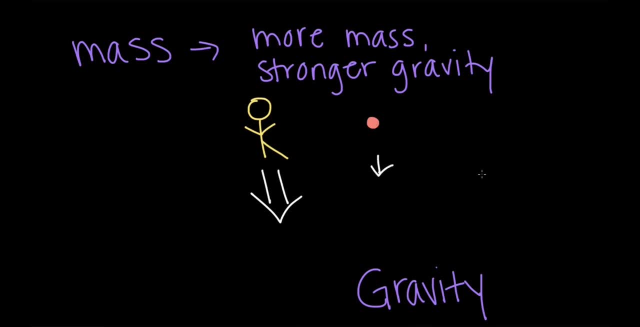 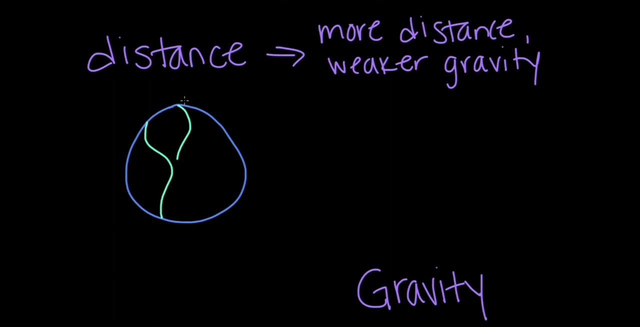 of gravity between a ball and the Earth, And that's why it's a lot harder to throw you into the air than a ball. Gravity also depends on the distance between the centers of the objects. As the objects get farther apart, the strength of gravity decreases. For example, if there is a ball on top of Mount. 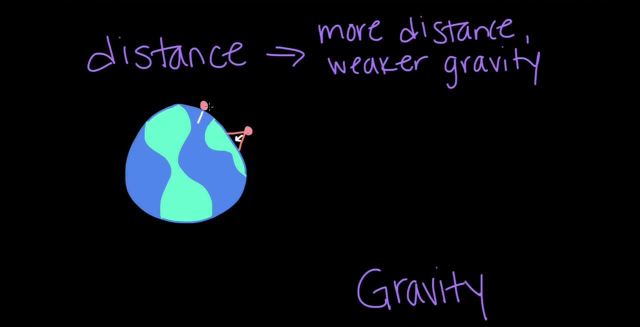 Everest, the pull of Earth's gravity on it is actually slightly less than the pull of gravity on that same ball at sea level, because the top of the mountain is farther away from the center of the Earth. Now this is a very small effect, less than a percent difference, because the difference between sea level 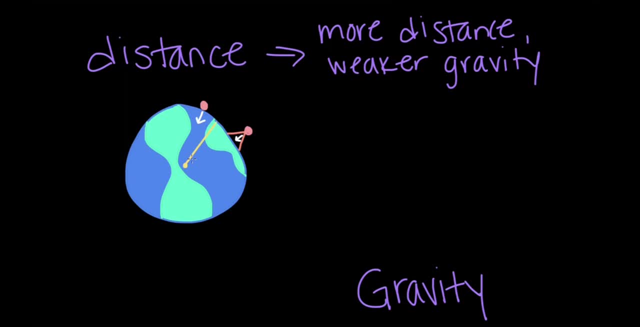 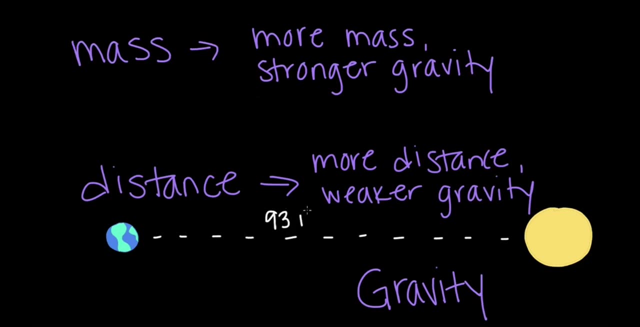 and mountaintop is still very small compared to the distance to the center of the Earth. But that's just on Earth. We know that things in space are really far apart. The Earth is almost 93 million miles, that's 150 million kilometers from the Sun. So if gravity is weaker when objects are farther apart, 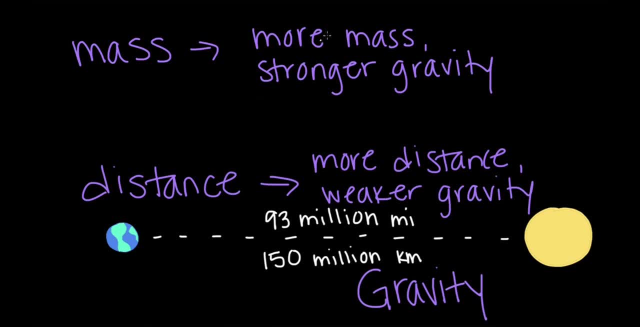 then, in order for gravity to be keeping these structures bound together, they must be really massive, And they are. The Sun has a mass of about 2 nonillion kilograms, that's 10 to the power of 30. And the Milky Way Galaxy, which is about a quintillion kilometers in diameter. 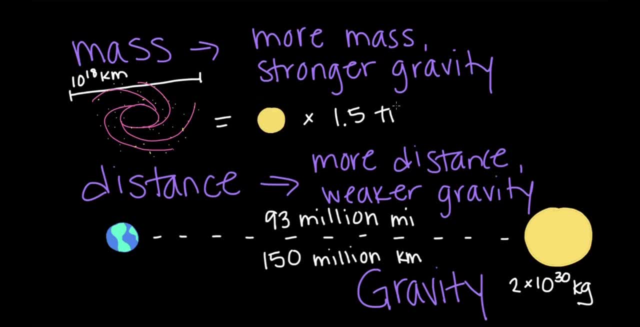 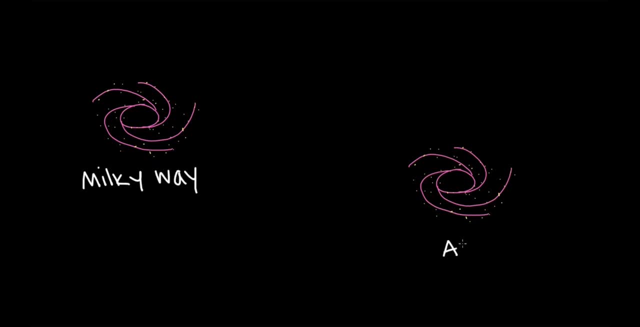 has a mass of about 1.5 trillion times that of the Sun. So, thanks to their high masses, objects like our Milky Way Galaxy and our nearest neighbor, the Andromeda Galaxy, which are the two largest galaxies in the local group, can be pulled together.